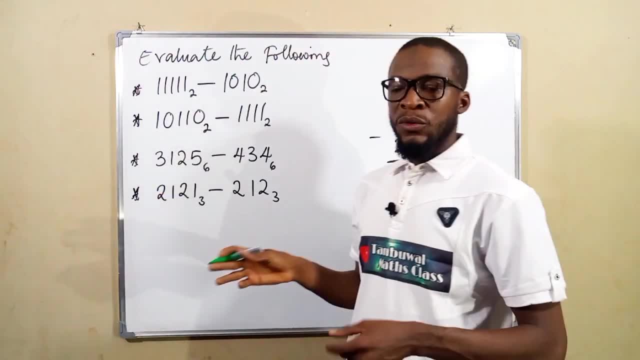 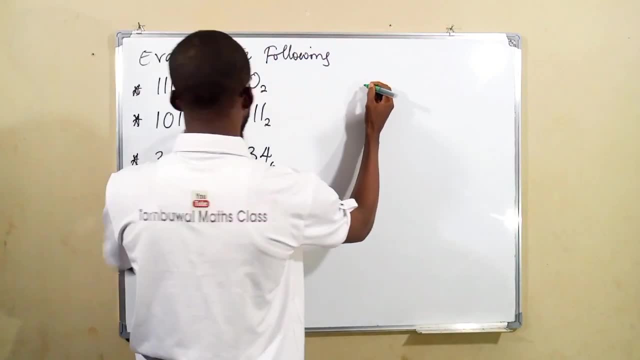 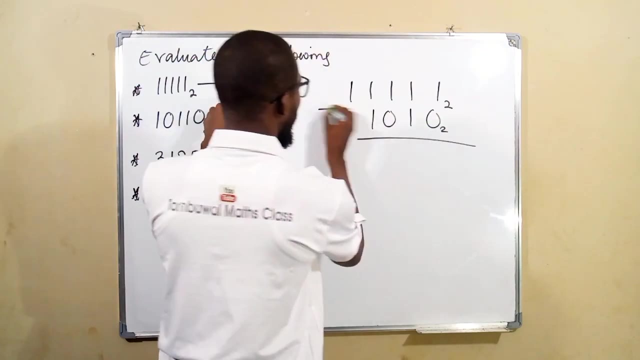 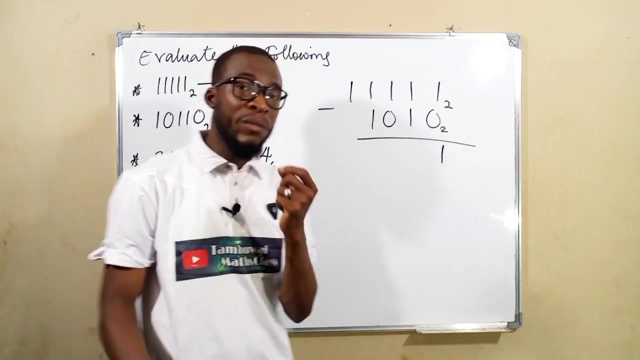 same principle is also applicable here. So now let us see how we can deal with these four problems. We are asked to subtract 1010 from 11111.. This is subtraction. We start from the right. One minus zero is one. I remember something: We can never have two in this set of numbers. 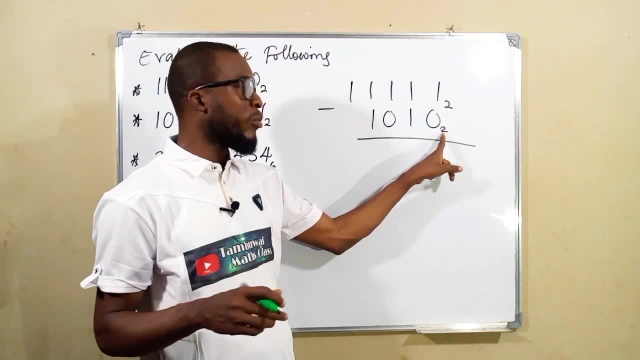 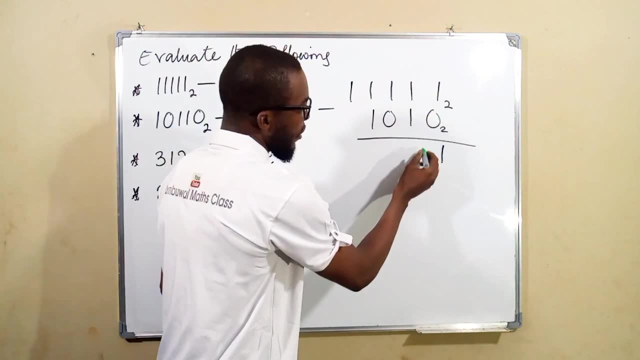 because the highest digit we can have is one less than the base. Our base is two, So the highest number is going to be one. Take note of that. We have: one minus one equals zero. One minus zero is one. One minus one is zero. One minus. 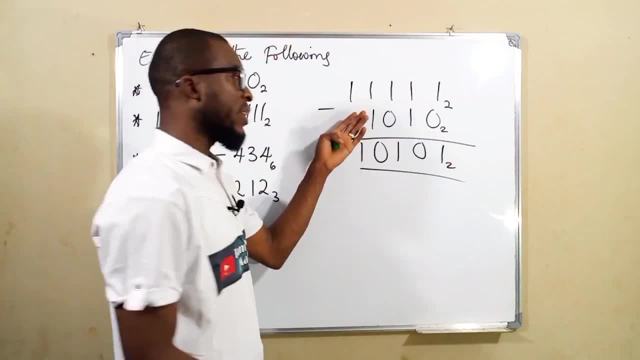 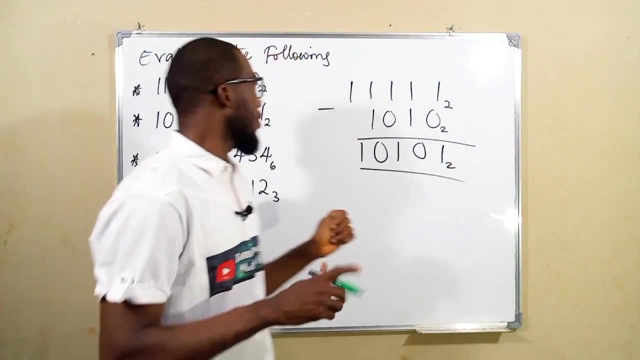 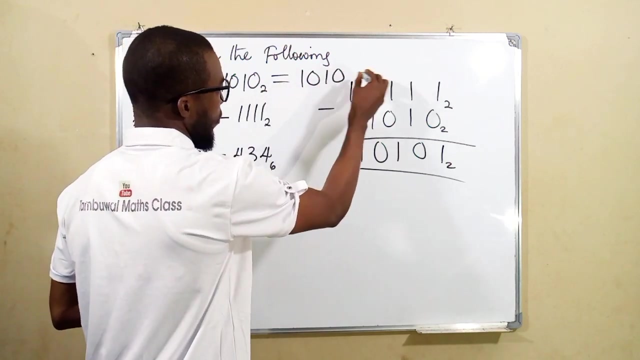 nothing is one. So this is what we have after subtracting 1010 from 111.. So this time around we have not borrowed anything. Now let us take the second question. Let me write this as 10101 in base 2.. So the next question: we are asked to subtract 1111 from 10110.. a subtraction: We are Bart conchita. a subtraction, Would you like to have a look? So the next question: we are asked to subtract 1111 from 110110.. 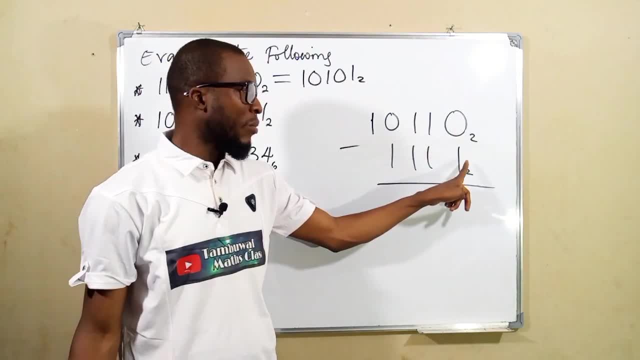 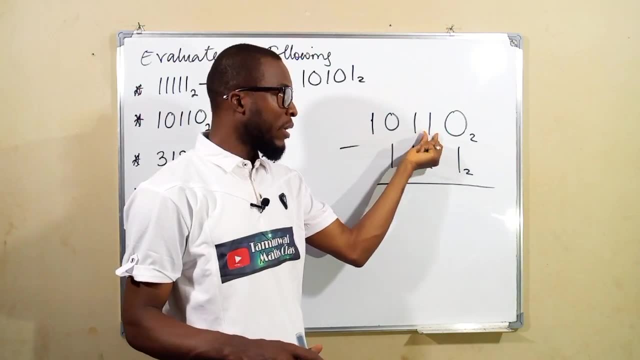 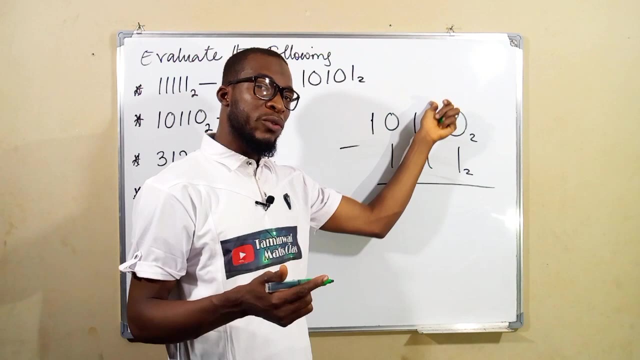 Subtraction. You can see here is zero minus one. We see it cannot be. We have to borrow one here. This is one bundle. Once this number reaches two It has to recount all over again from zero and take one bundle in the next So we can say if that one bundle should come. 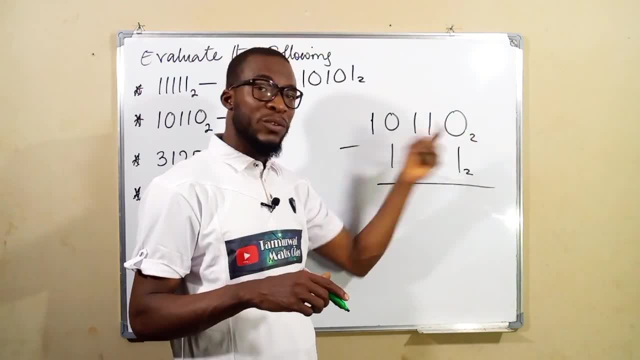 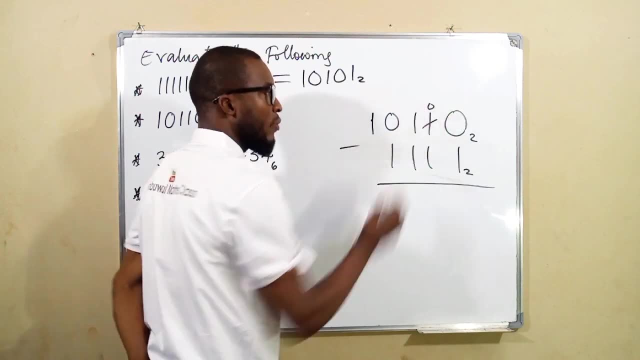 back. it is going to come back the next ring, So this subdruction will also consequentially as 2, because that's one bundle in base 2. so 0 minus 1, it can't we borrow one here. this one is no more, we have 0, but what is coming will come in term of our base. 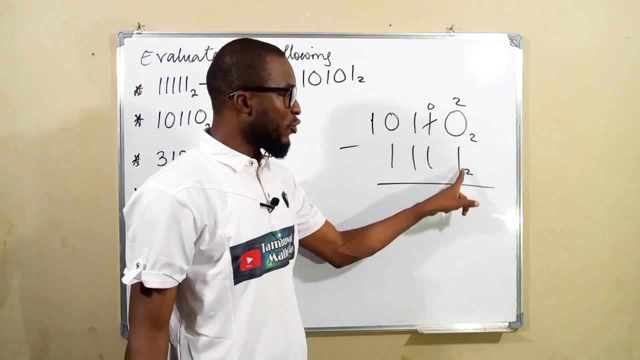 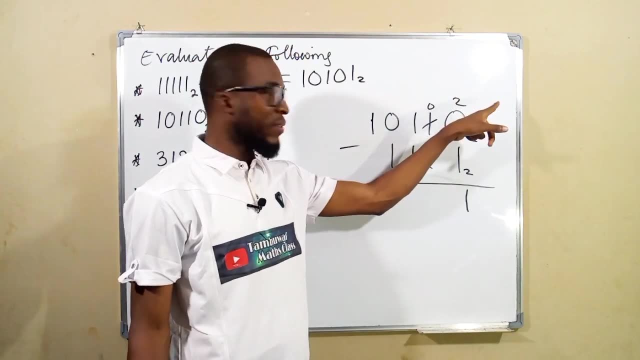 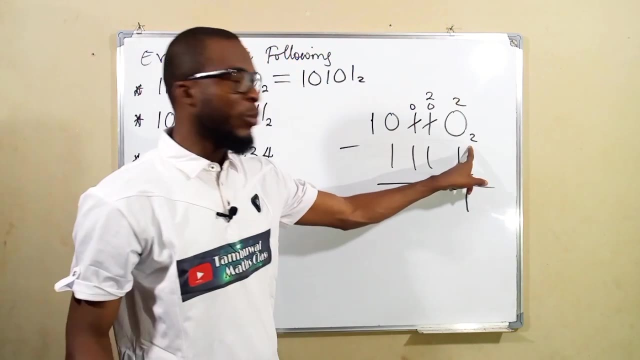 which is 2, 2 minus 1, is 1. here we have nothing because we have already taken away the bundle to the next. we have to re-borrow here again. this becomes 0 and whatever number is coming, it will come in term of the base, which is 2, 2 plus 0. 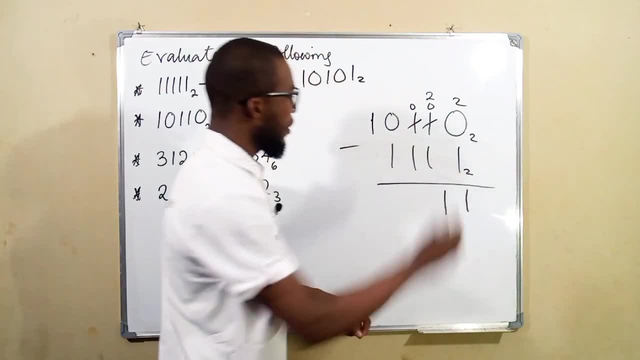 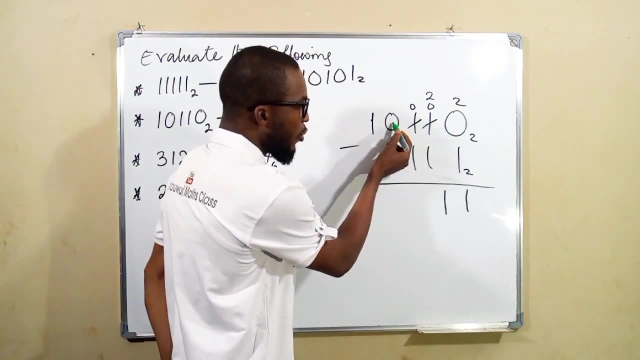 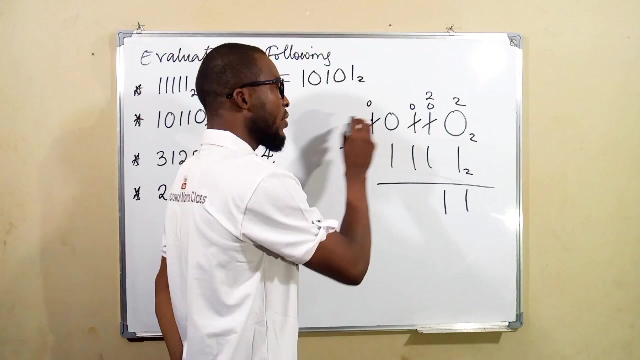 is still 2. 2 minus 1 is 1. again here we have nothing, but we have 1 under. we want to subtract. we are not going to borrow here because this one has nothing. we are going to borrow here. you take away one bundle here you are left with 0. you. 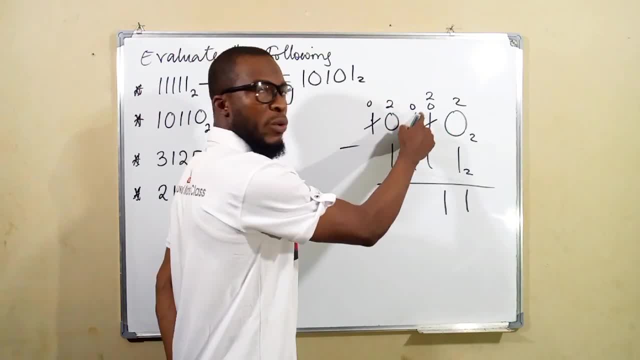 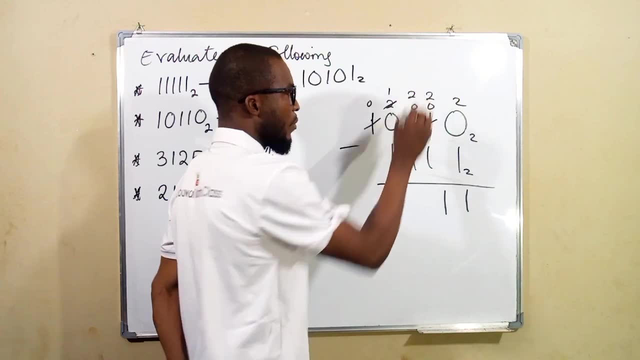 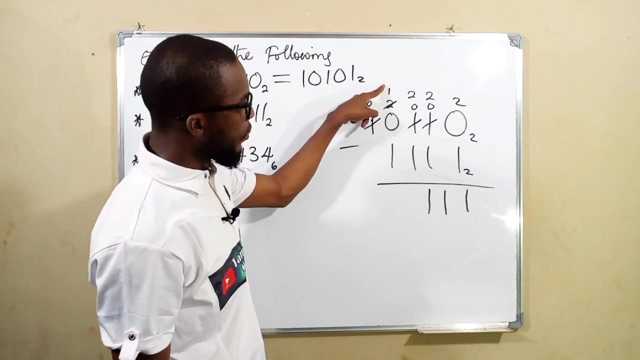 bring it here as our base. but this is where we want to bring the bundle. take one bundle here, leaving one bundle. bring the other bundle back here. it becomes 2. so 2 plus 0 is still 2. then 2 minus 1 is 1. here we have 1 left, 1 minus. 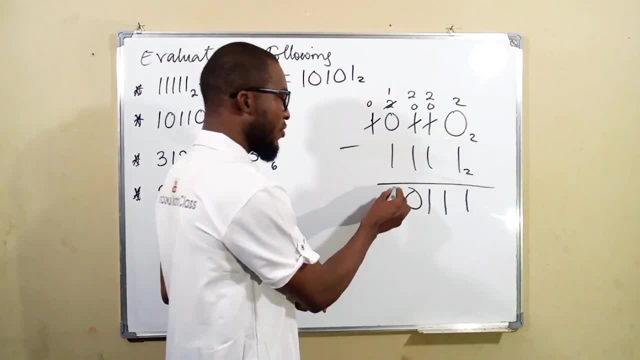 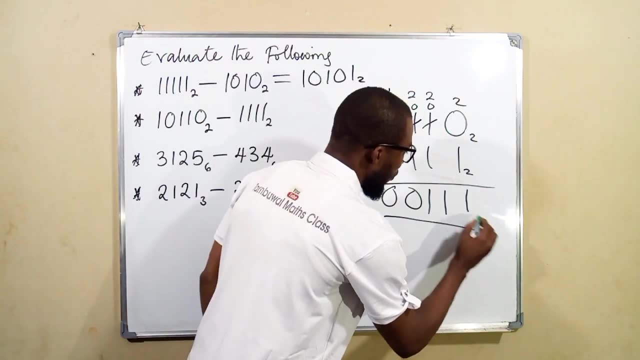 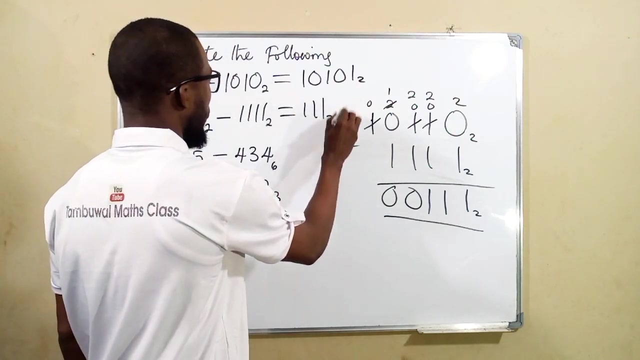 1 is 0, but here we have nothing. nothing minus nothing is nothing. so these two zeros are not significant. if you like, you leave them, if you don't, you remove them out. So this is what we have in base 2.. 1, 1, 1.. So you can write it here: 1, 1, 1.. Also in base 2.. 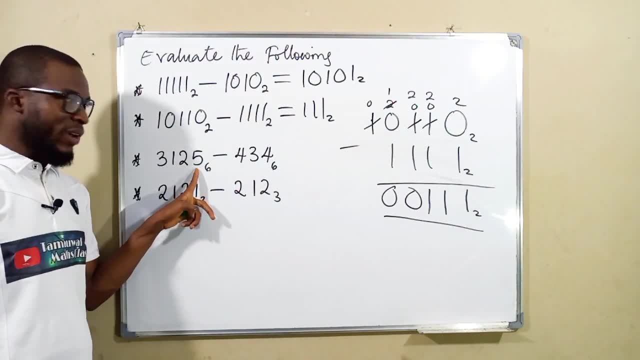 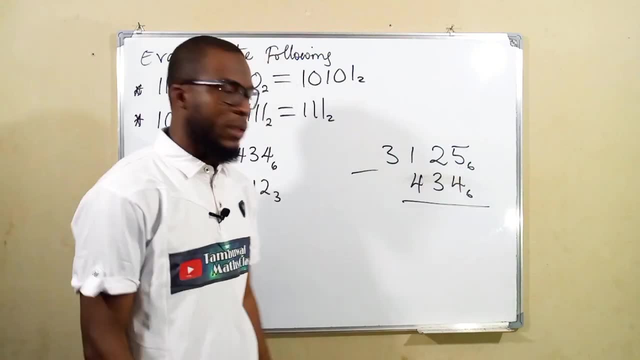 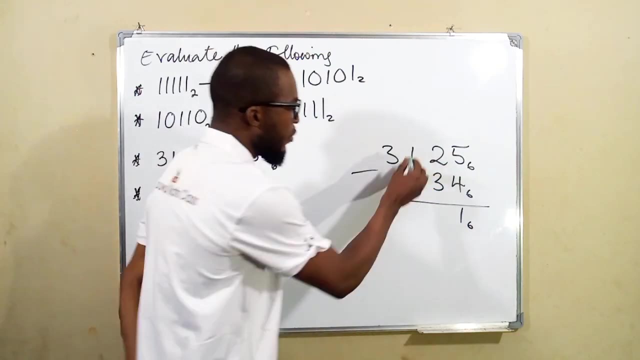 Here we have numbers in base 6.. The highest digit we have is 5.. You can see, We will never have 6 here. 5 minus 4 is 1.. This number is in base 6.. 2 minus 3: we have to borrow. We borrow here. 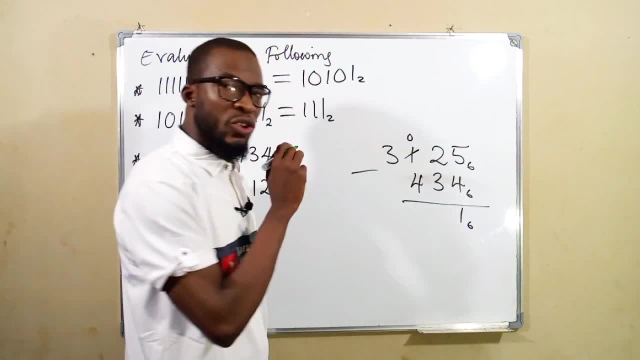 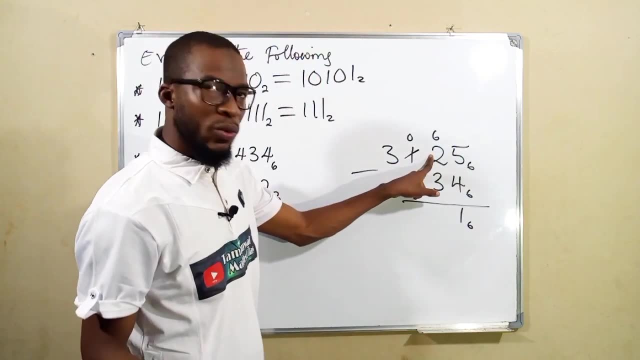 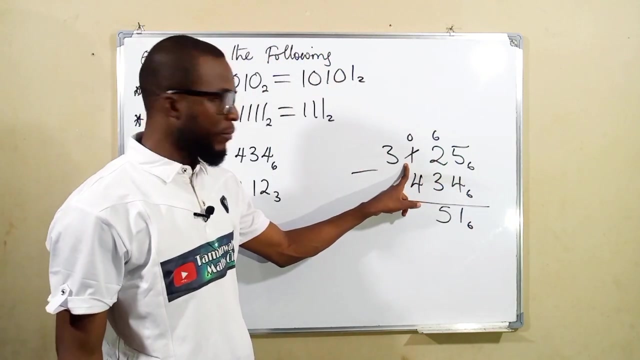 This is one bundle. We are left with nothing. Once it comes here, it will come as 6.. So you see, 6 plus 2 is 8.. Then that 8 minus 3 is 5.. So we have 5 here. We have nothing here. 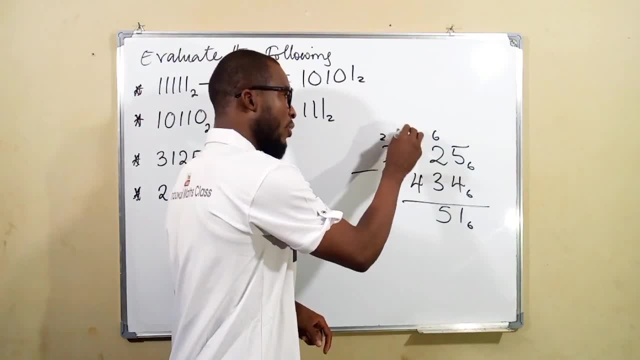 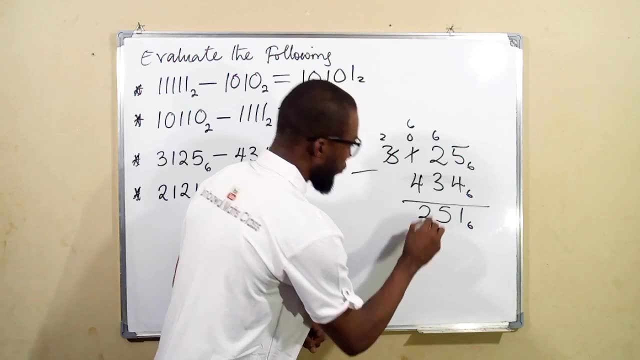 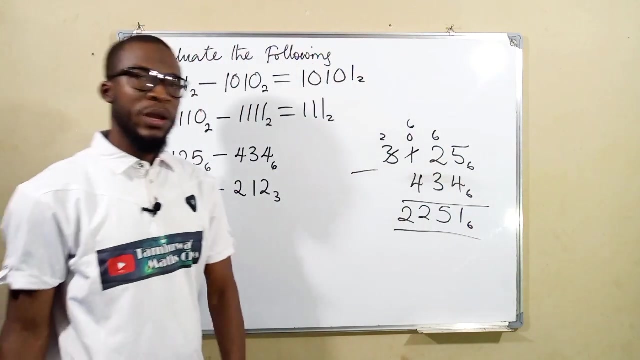 So we borrow one bundle here, leaving two bundles. What you are going to bring here is 6.. 6 plus 0 is still 6.. Then 6 minus 4 is 2.. Here we have: We have two bundles Minus nothing is still 2.. So this is what you have: 2,, 2,, 5, 1.. 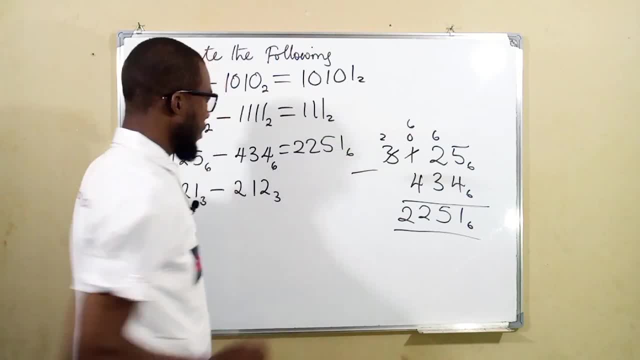 2, 2, 5, 1 in base 6.. Okay, let us look on to the last one, which is 2, 1, 2, 1 minus 2, 1, 2 in base 3.. 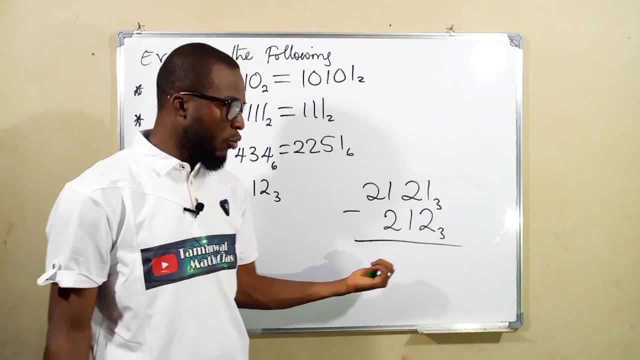 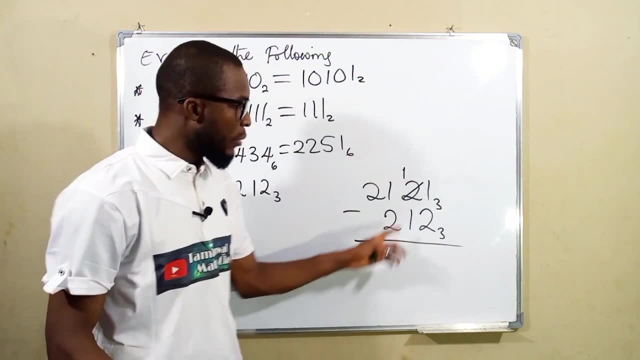 We start from the right. 1 minus 2, it can't We borrow 1.. This is two bundles. We are taking one bundle away, Leaving a single bundle, But that bundle will come here as 3, which is our base. 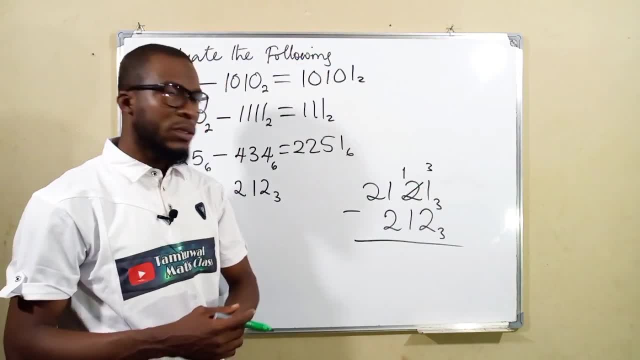 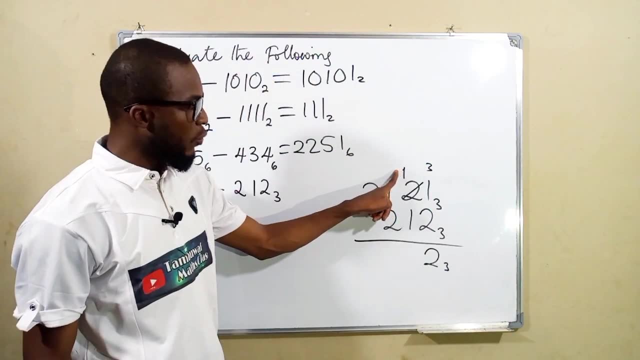 So we have 3 here. So 3 plus 1 is 4.. Then 4 minus 2 is 2 in base 3.. Here we have one bundle left. 1 minus 1 is 0.. 1 minus 2: we have to borrow again.